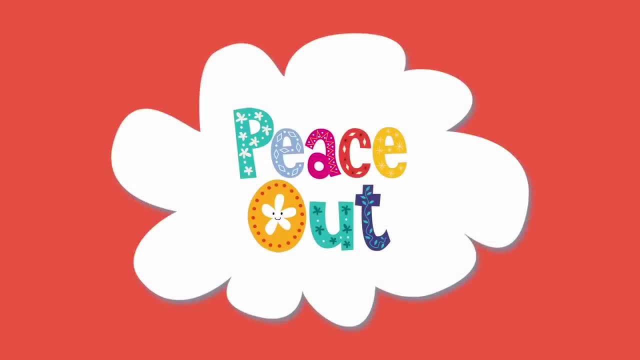 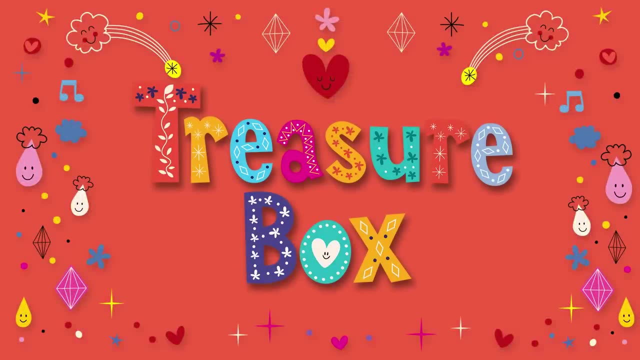 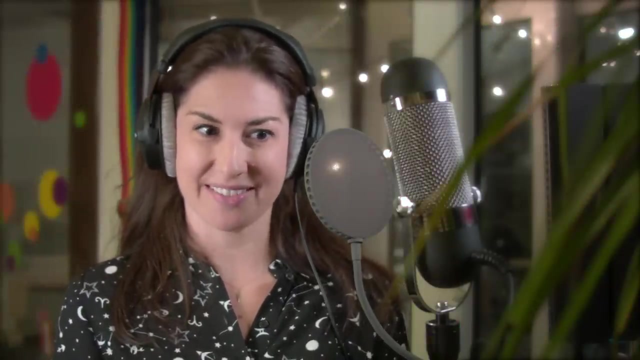 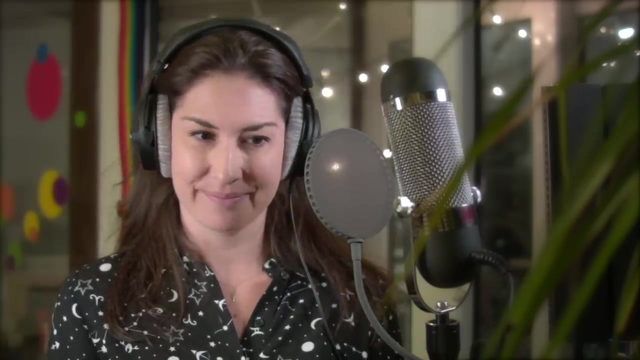 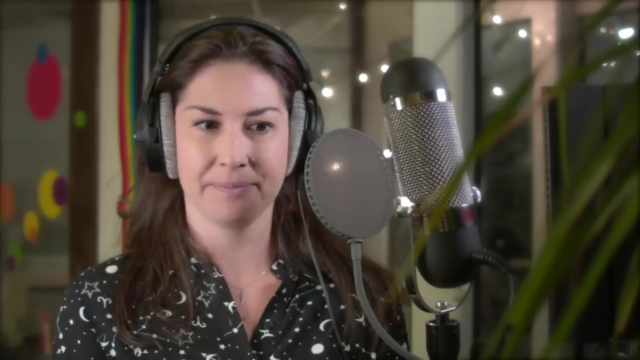 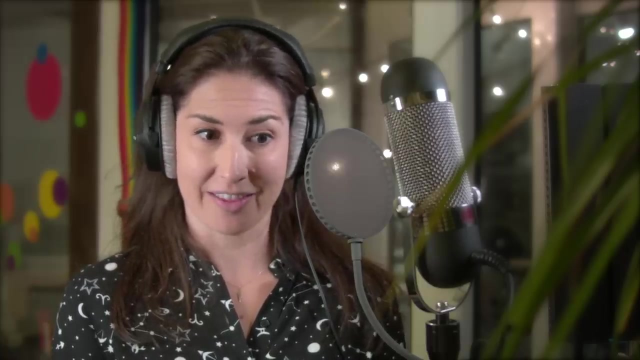 Hello Jamie here. Welcome to Peace Out. Let's get ready by finding a place to sit down or lie back. Get yourself really comfy, making sure you feel snug and warm Once you're settled. let's begin by tuning into our breath. We always do this, as it helps our body relax. 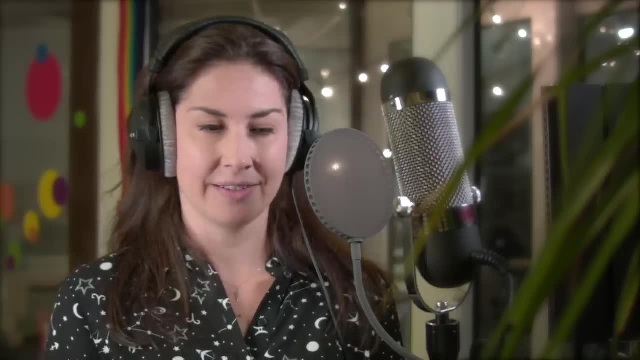 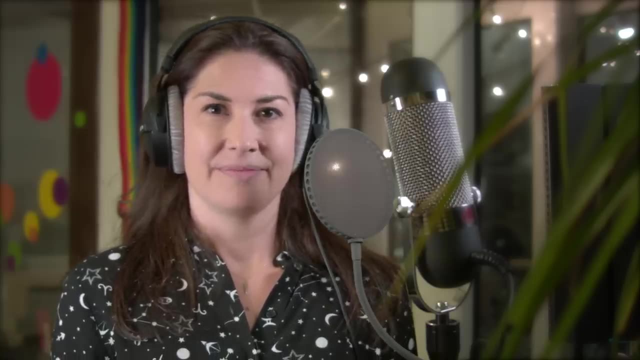 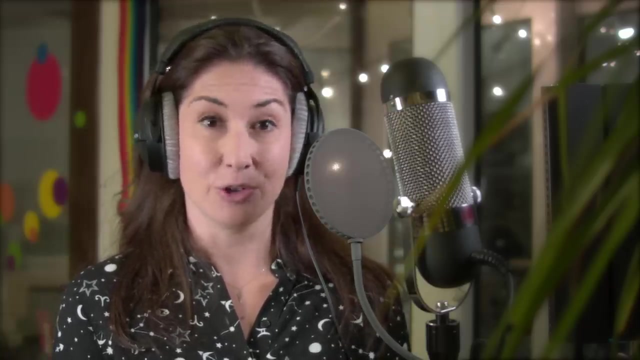 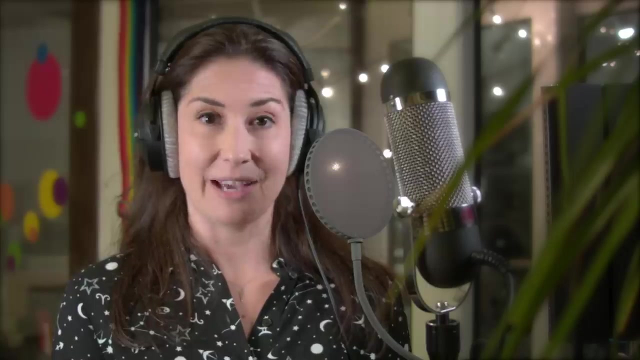 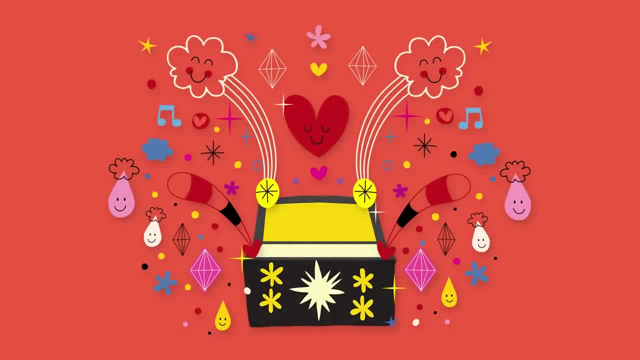 and our mind feel clear. See if you can notice your breath Coming in and going out. Feel the coolness of the air on your nose as you breathe, If you haven't already allow your eyes to gently close so you can go inside for a bit Now. 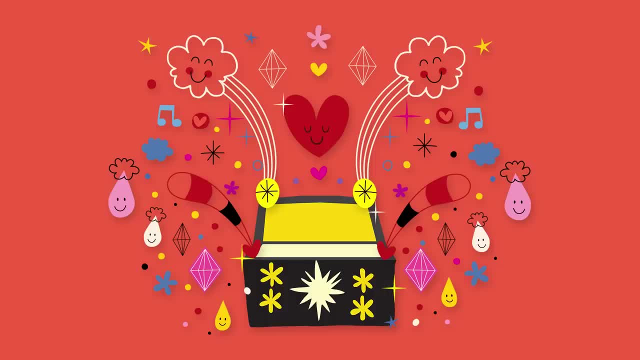 imagine there's a little balloon just below your bed. As you breathe in, the balloon blows up a little And as you breathe out it goes flat again. Slowly breathe and enjoy the feeling of your balloon filling up, then emptying out. Breathing in, filling up, Breathing out, letting it empty. 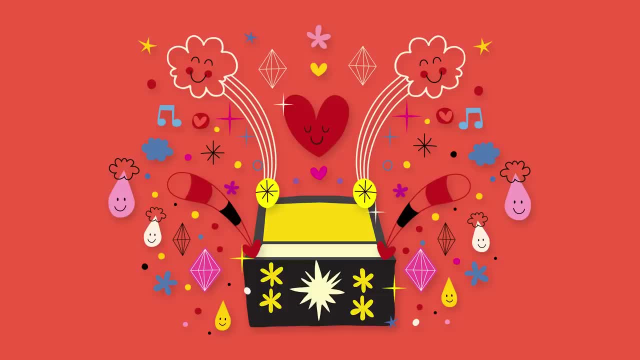 Well done. Now see if you can imagine a place, a special place that is all yours. This is a place where you feel relaxed, You feel safe here and happy. It could be a room inside a cozy house, a meadow, a forest. 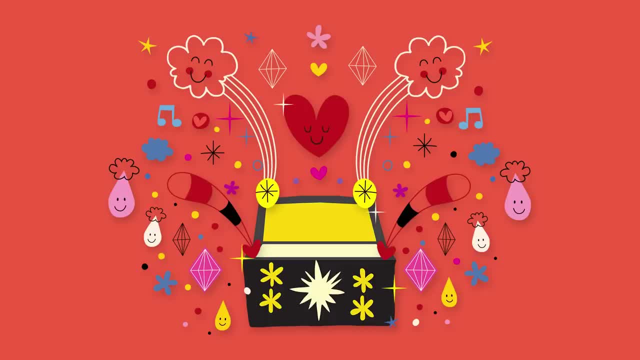 Or on a beach, Wherever it is. go there now in your mind, See yourself in that place right now. Look around. What can you see? What colors are around you? Blue, orange, pink, purple, blue, blue, pink, blue, blue. blue, blue, blue. We're in a mango, aren't we? We're in a mango As we get older. we're in a mango. It's like a mango that only Joe and I can see. Oh, it's like a little bird. We're in a small house. 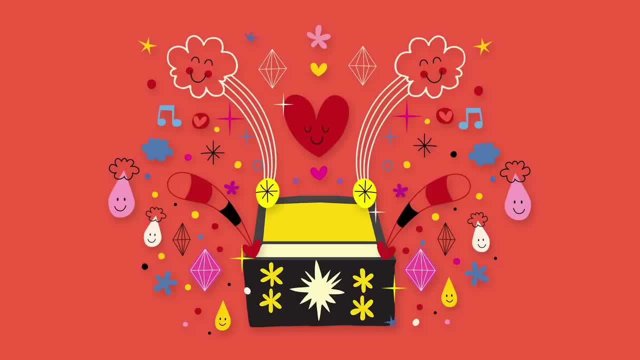 yellow. Take them all in. Can you hear any sounds? Birds chirping, The wind blowing gently, Ocean waves, A fire crackling. Listen for the sounds. You touch something and notice how it feels. Is it cool or warm Here in your place? you? 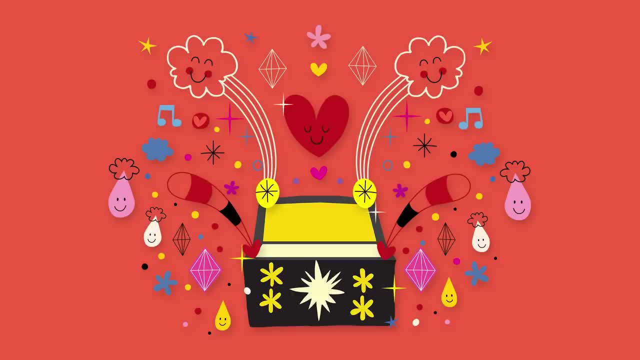 feel totally peaceful, happy and safe. You smile to yourself enjoying your special world, A safe place you can come to wherever you need A safe place. you can come to whenever you need. Here in your place, you have an animal friend. You decide what. 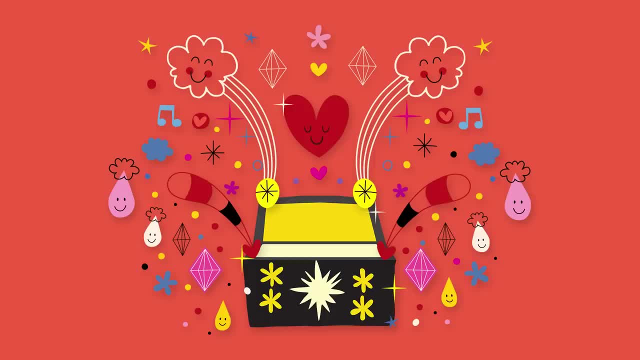 sort of animal you'd like your friend to be. It can be any animal you like. See if you can imagine it. now It's coming over to you to say hello. You feel very happy to see your animal friend here and follow it, as it seems to be your. 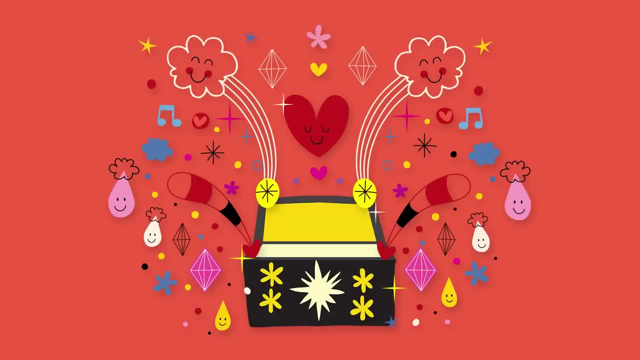 friend. It seems to want to show you something. There's a tree and leaning against the tree is a shovel, a spade. Your animal friend is very excited and suggests you start digging beneath the tree. Your friend helps you to dig and uncover a. 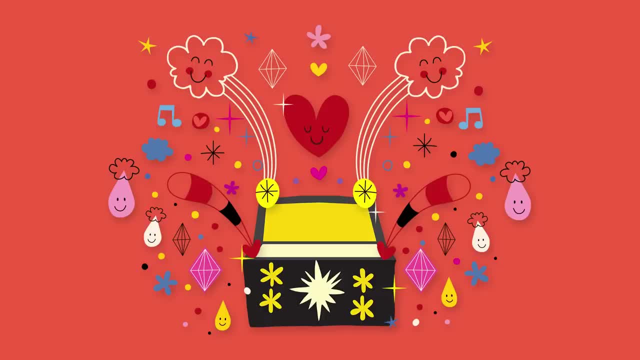 black treasure box covered in sparkling jewels. Attached to the box is the key, So you open it. Inside are some of the most special things: Photos of you having the most amazing time, The people you love most in your life, Your favourite snack And a note written to you. 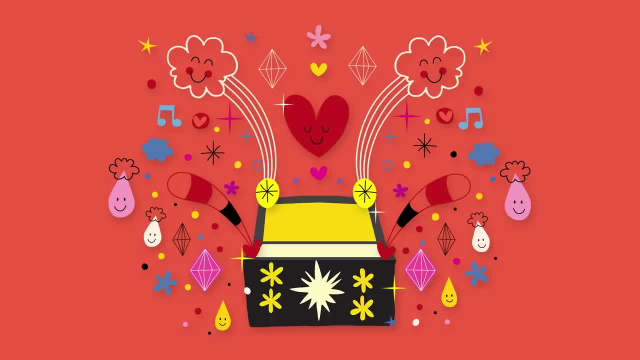 from your very own heart. Put it in your shoulder. There's a own heart. The letter says that you are deeply loved by your family and your friends. You should just expect people to be nice. You don't need to worry about kids who are mean And 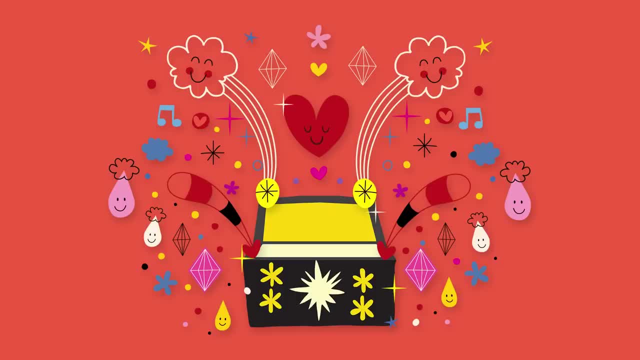 most importantly, Love yourself. Love yourself as you sit there with your animal friend. You take in these words that come from your very own heart. love myself, Yes, you can do this. You look up at the sky and it fills with colour, the colour of love. You decide what colour that is. You breathe your colour in and out And as you, 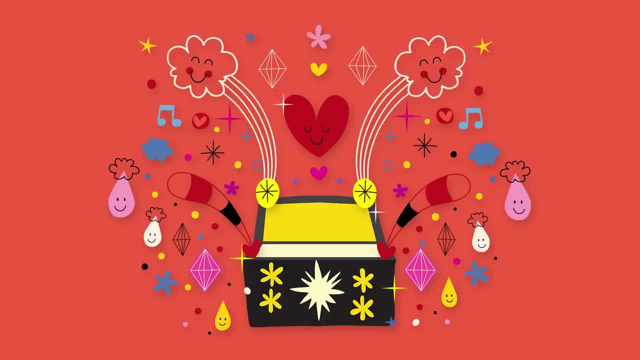 do you feel love filling your heart With each breath. more and more your heart fills As it does. you forgive yourself for being hard on yourself, for saying negative things to yourself, for not being perfect. You have opened the door to love in your heart Now. 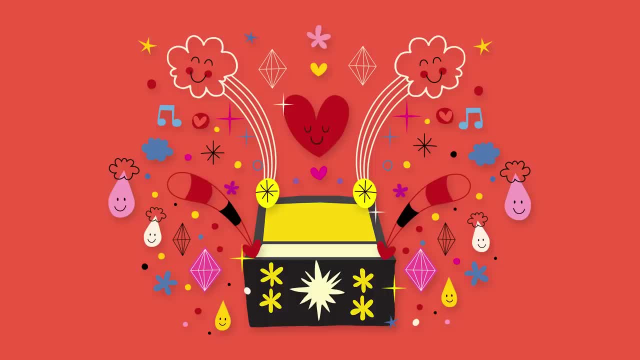 you can receive love and give love. Take that with you. Fill yourself with love, Listen to your heart and expect people to be nice. Slowly, now we begin to come back from this magical place, saying goodbye to our special animal friend, giving them a hug. 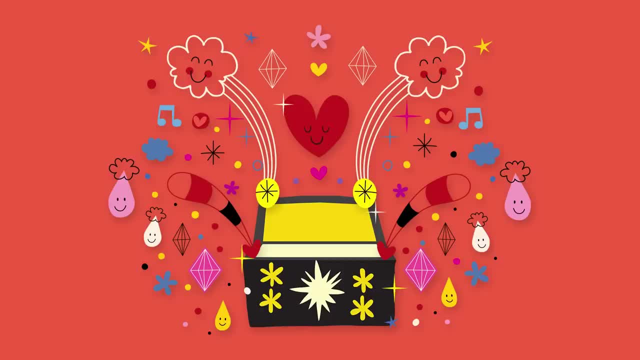 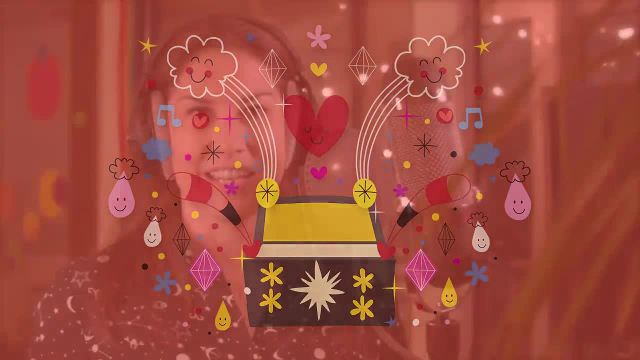 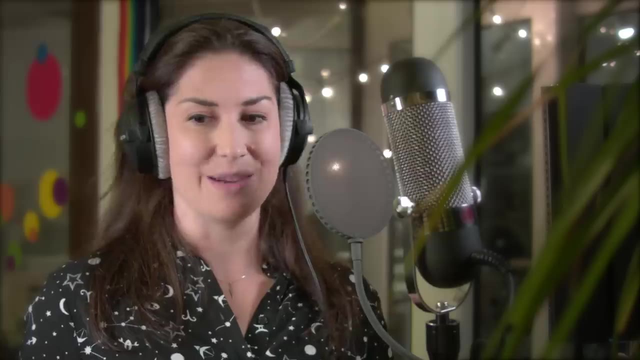 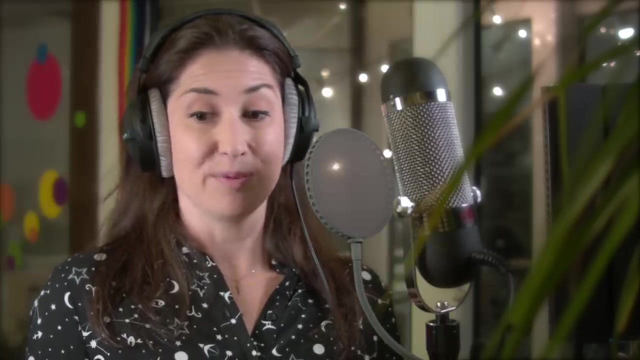 and feeling them hug you back. We wiggle our fingers and our toes and we gently open our eyes. Take a moment here, before you move anywhere, to just notice the feeling you have inside you now. Hopefully, you can still feel that sense of love in your heart and enjoy. 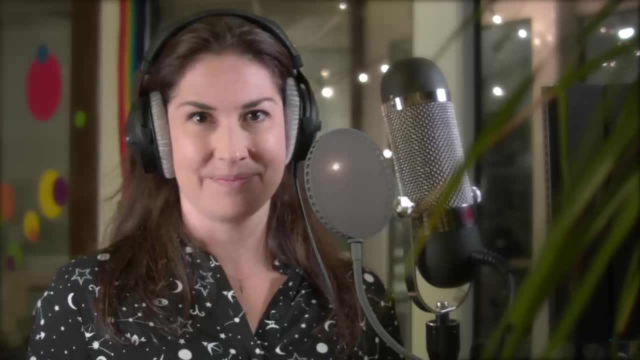 taking it with you into your day. This is Jamie saying peace out.